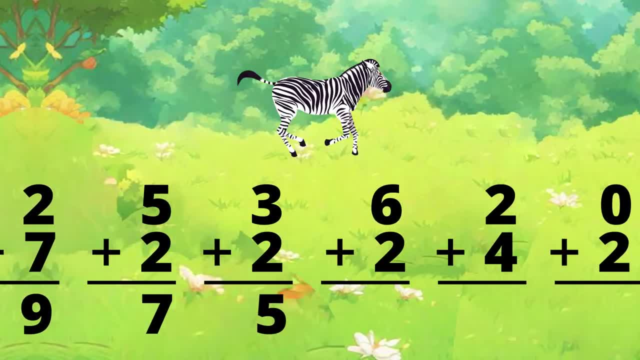 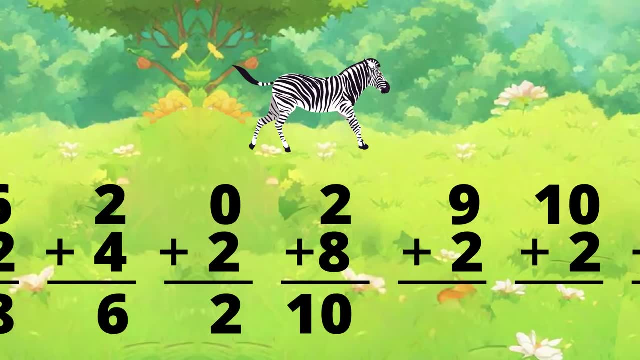 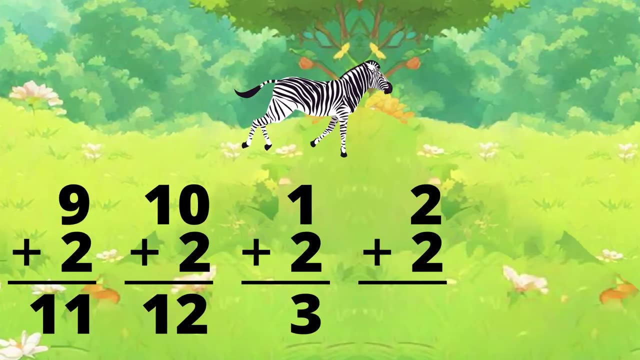 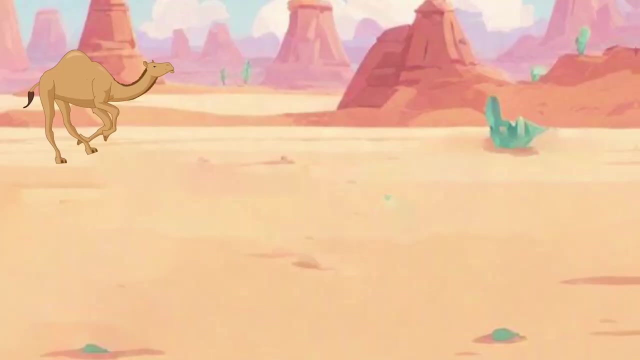 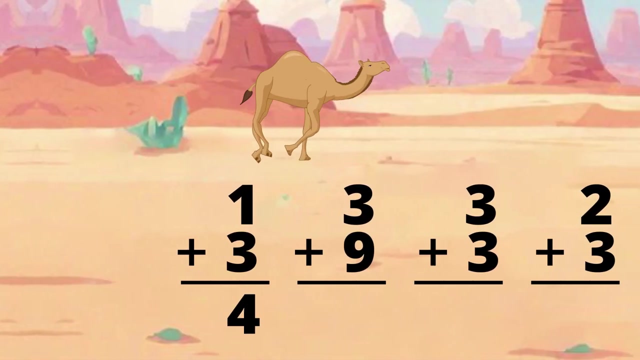 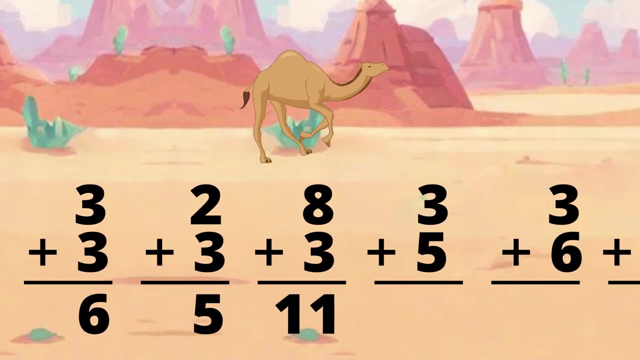 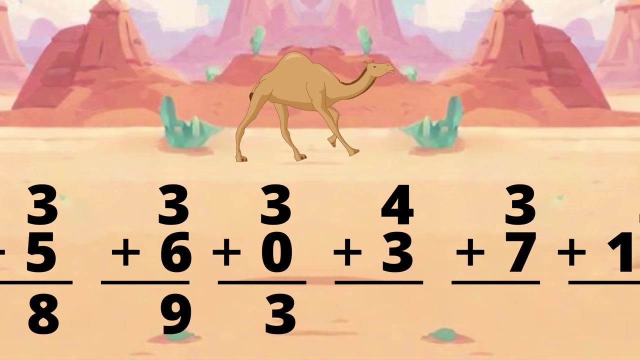 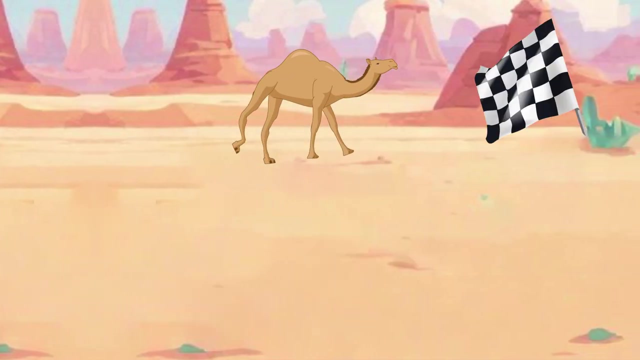 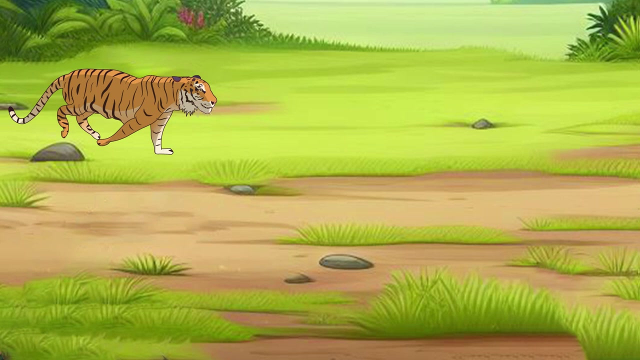 How did you do? Did you beat the zebra? Now we'll add threes. Can you beat the camel? Ready set go. How many did you get right? Now it's time for the fours Race: the tiger- Ready set go. 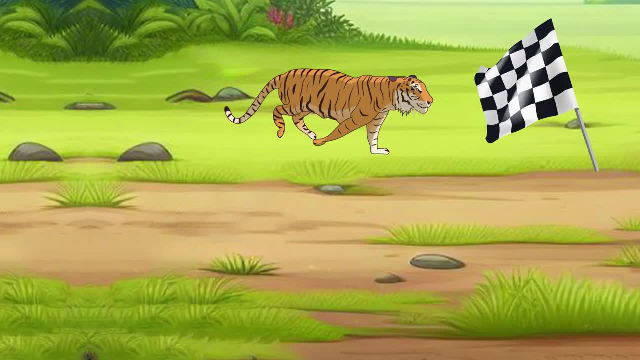 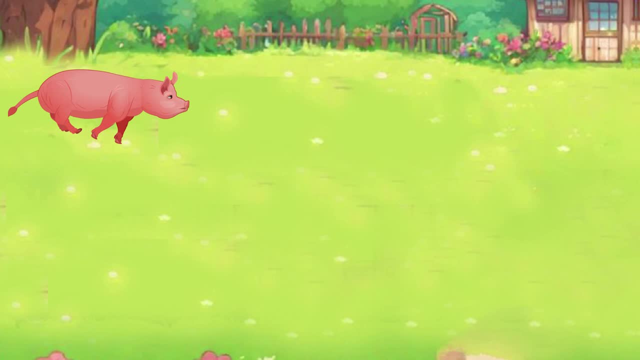 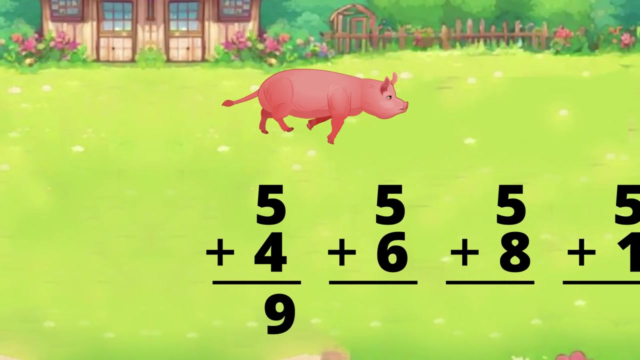 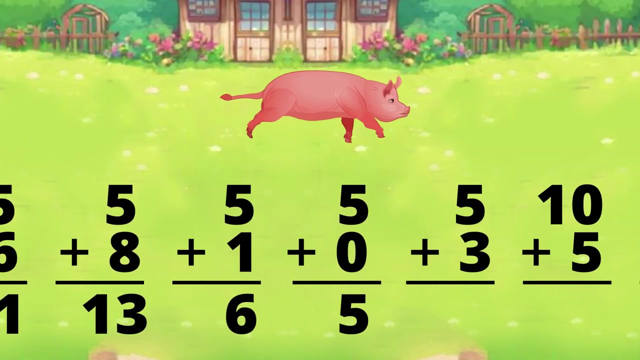 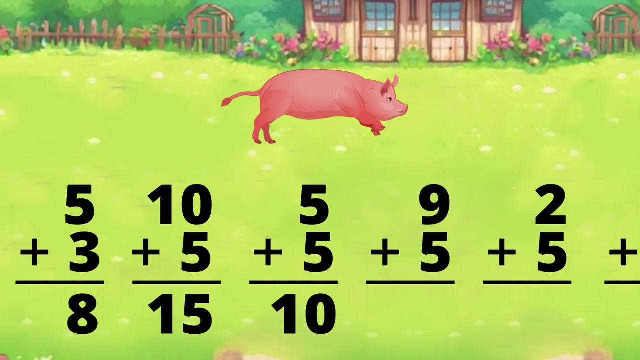 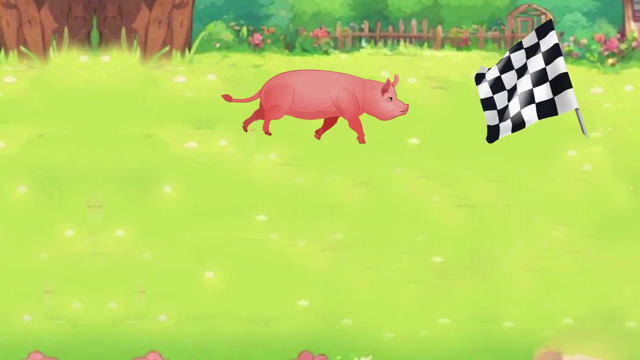 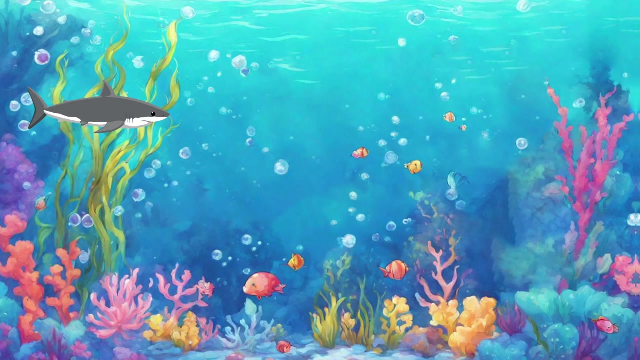 Did you win? Next you'll race through the fives against the pig Ready set go. Were you faster than the pig? This race will test your knowledge of adding six. competing against the shark Ready set go. 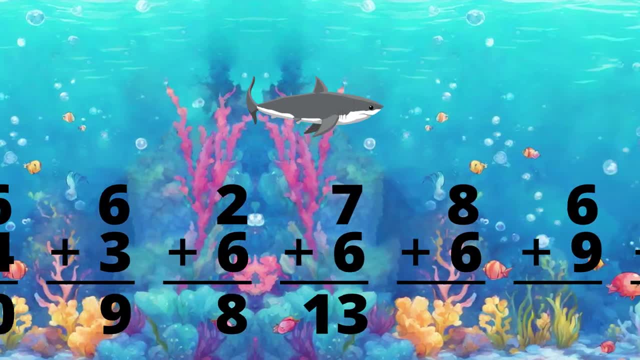 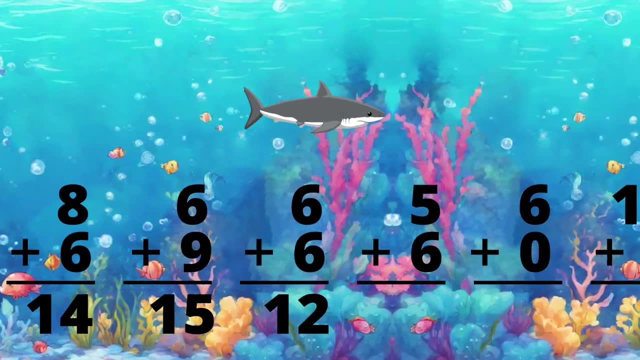 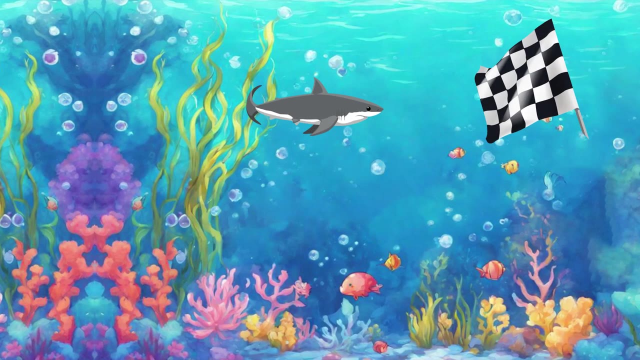 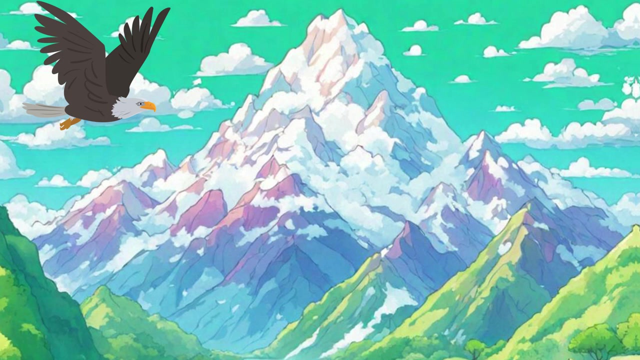 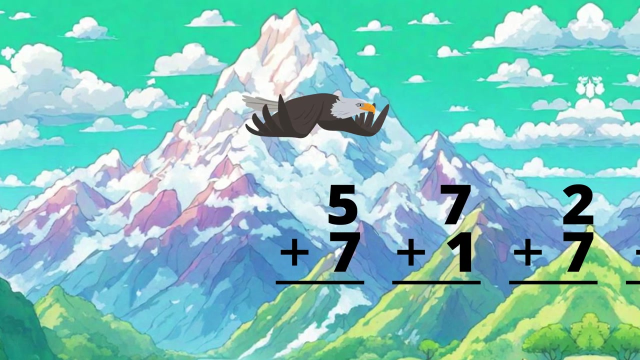 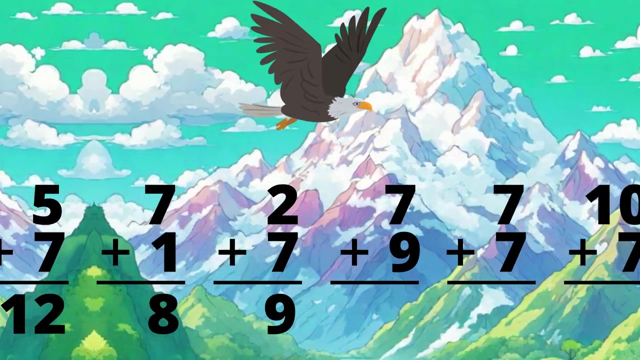 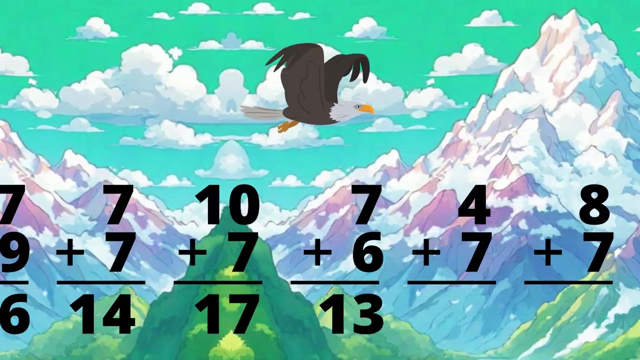 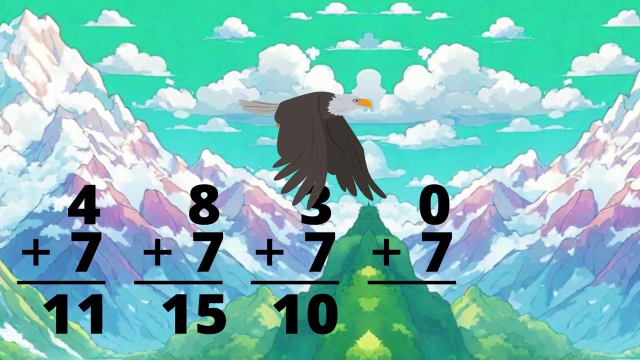 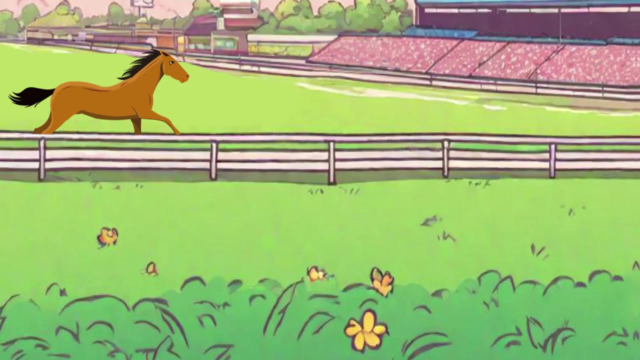 How did you do Get ready to race against the eagle to test your knowledge of the sevens math facts? Ready set go, Ready set go. Did you get the answers before the eagle did? Now we'll race over the eights with the horse. 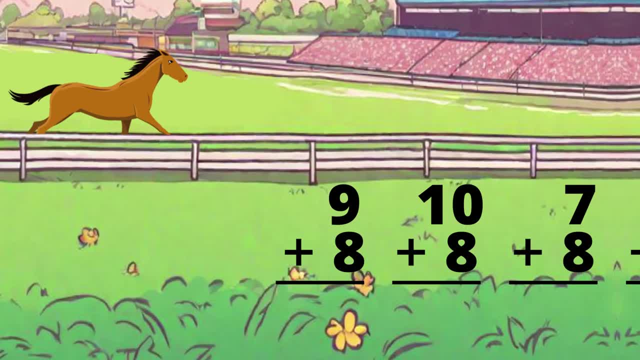 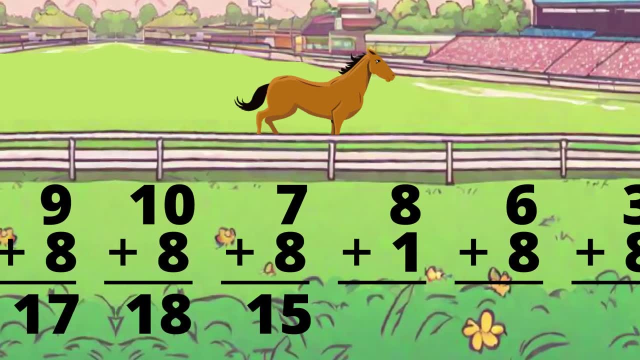 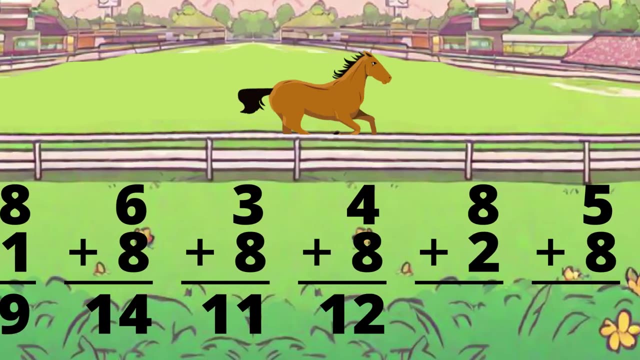 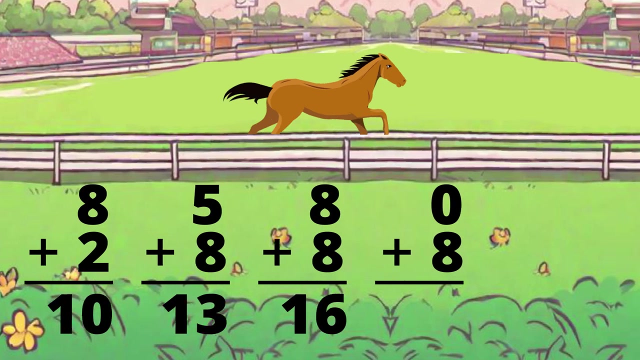 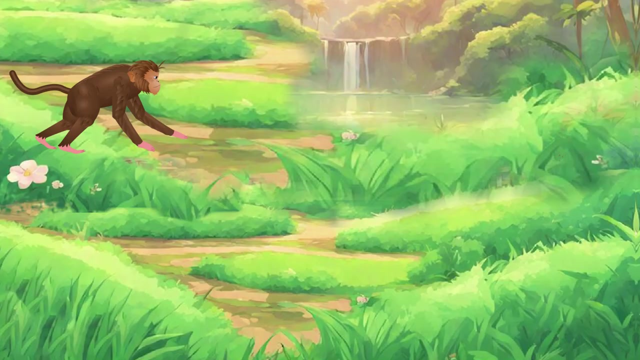 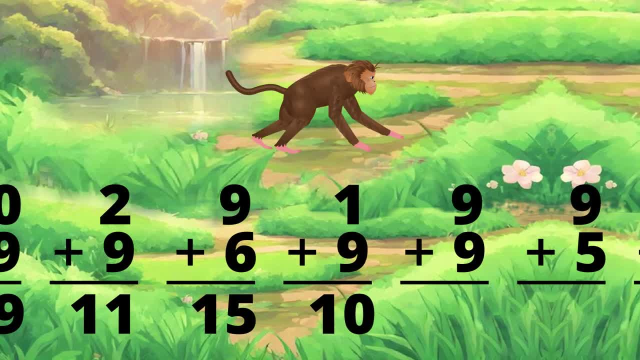 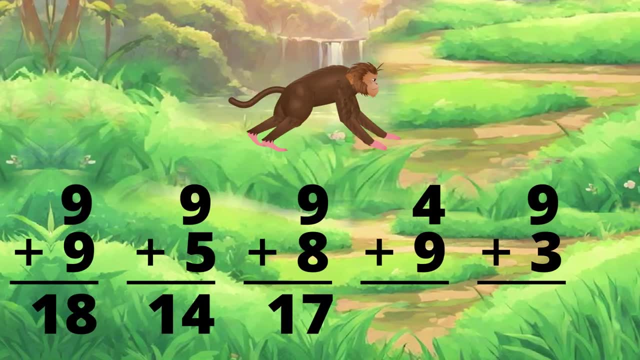 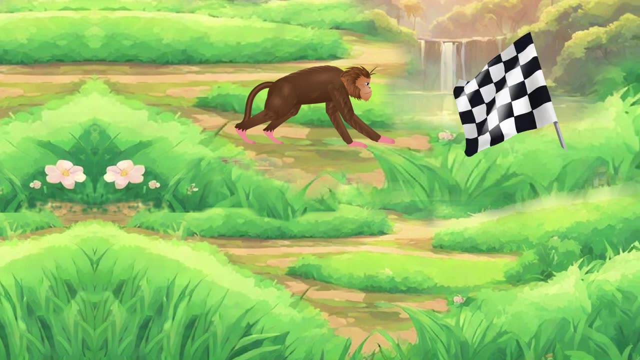 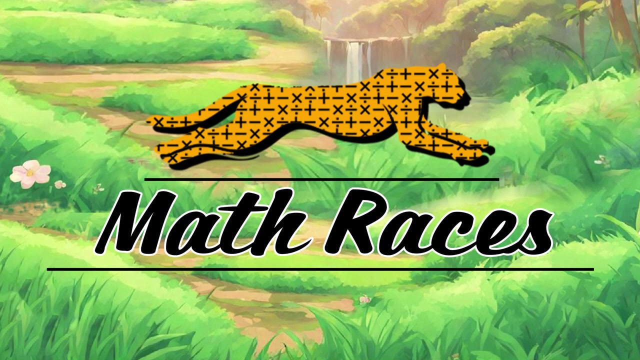 how did you do on your nines? if you didn't do well in some of the races, you can always come back to this video and try doing these math races again. 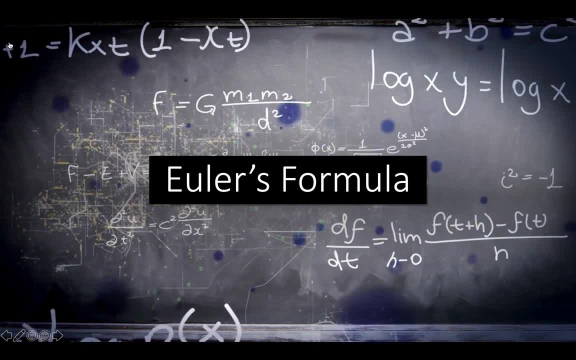 For my presentation I chose to do Euler's formula, which is a beautiful formula from 3D geometry about polyhedra. I'm going to start this presentation off by explaining why I chose the topic. I'll then move in to what the formula actually means. What does it describe about 3D? 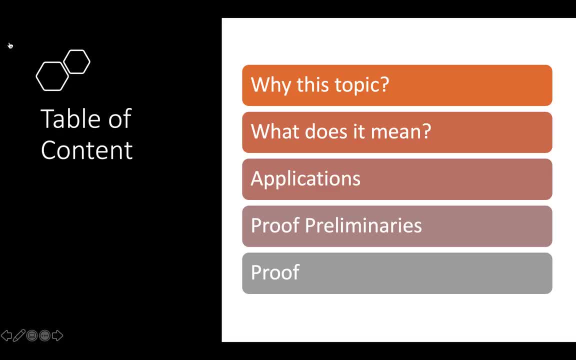 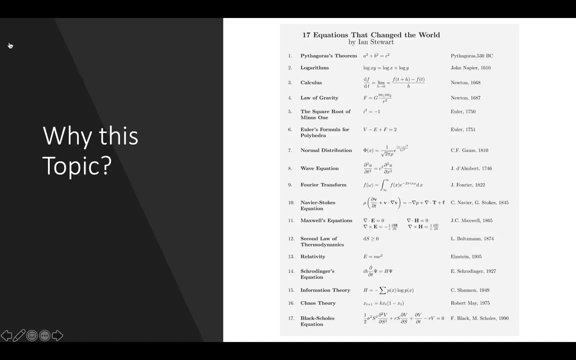 geometry and polyhedra. We'll then move into applications and I'll run through some examples and then straight into proof preliminaries and then on to the proof. So if you spend any time online in math blogs or on Twitter, if you follow some mathematicians- 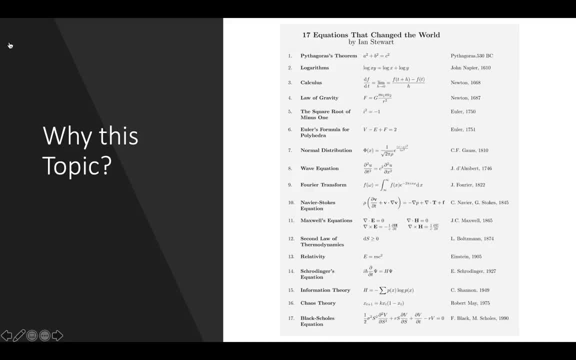 occasionally they'll share a list of the most famous equations or their favorite equations. So this is a list by Ian Stewart, somebody I follow on Twitter, and he just shared a list of a bunch of famous equations, And you'll notice that equation number six is Euler's formula for 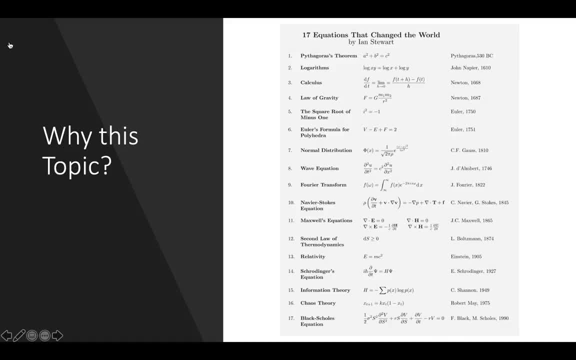 polyhedra. I've never been in a class where I learned about the formula, So I just wanted to know why it's so famous. So I just wanted to take this opportunity to dive into the details and understand what the formula says and how it's proved. What does the formula mean? Well, here we have a collection, a random